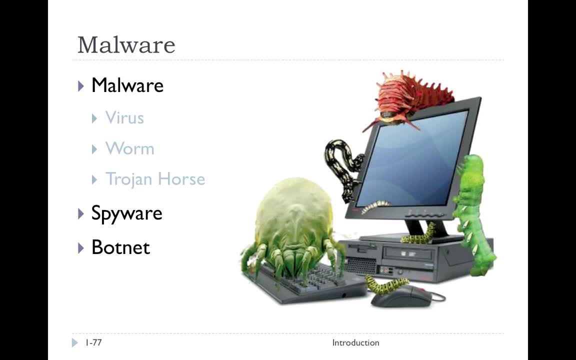 um are bad software: Viruses, worms, trojan horses, um. each of these pieces of software will may infect a host, a computer, and do bad things. The um, a trojan horse, is a hidden part of some otherwise useful software. 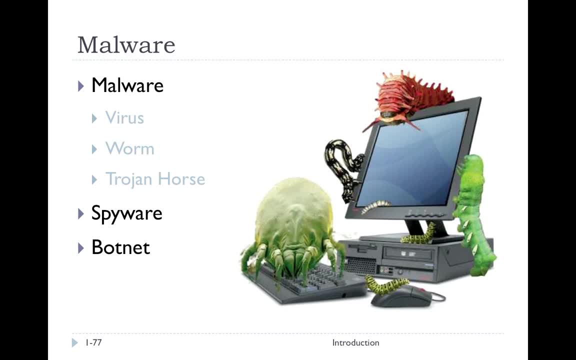 um that will sneak into your, your system. A virus is an infection that's received by an object, often an email attachment or some downloaded downloaded program. It typically involves um a self-replication process, where it will propagate itself to other hosts and other users. 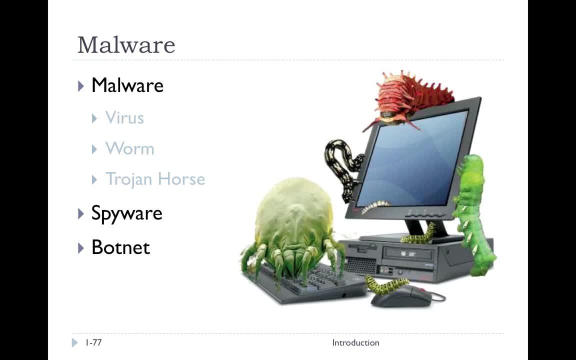 um by expanding and pushing itself out. A worm is an infection that's passively received um and gets itself exe executed. It will also be self-replicating. There are types of other types of malware, include spyware. 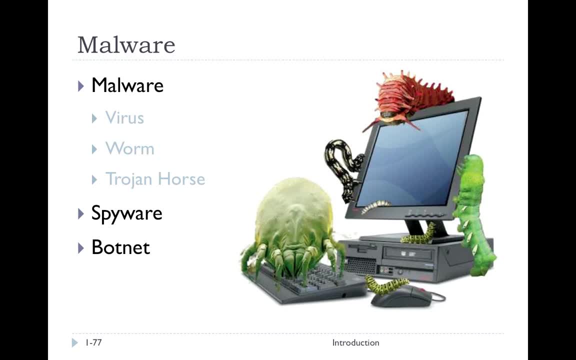 which is software that might kind of spy on user activities, Like keystrokes or websites visited um those sorts of things to collect information behind your back. When infected hosts are kind of grouped together- and a lot of hosts have been compromised, those that group of collected hosts can be used as a botnet. 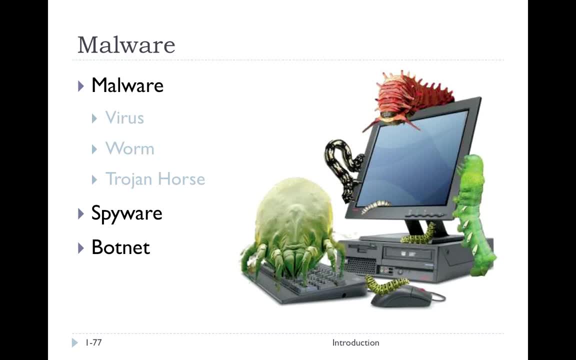 and used for spam and denial of service attacks, especially distributed denial of services attacks. Um, so there's lots of types of malware and we'll talk more about these um later on in uh the course. Um, this graph is from the author. 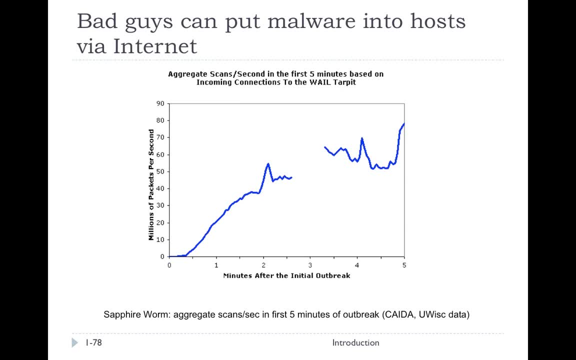 and it kind of shows you this old uh worm outbreak, the sapphire worm, and how quickly it sent a lot of packets. You see just minutes after the initial outbreak how many millions of packets per second were being sent out by this worm. 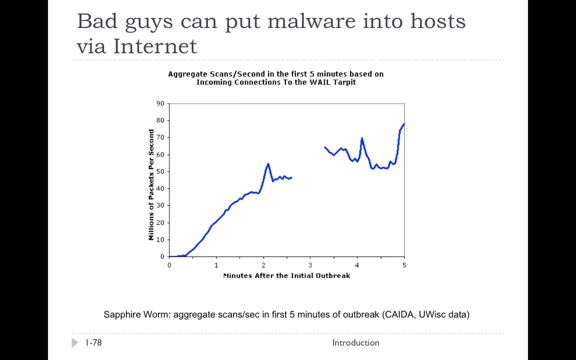 So, as um, as these worms and viruses, uh, because they're self-replicating, they can cause this exponential explosion in network traffic. um, if that's the thing they attack, Um, we're gonna look at some other types of uh. 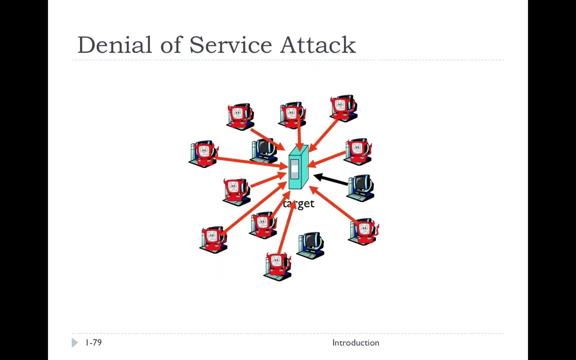 other types of attacks as well. One very popular attack is the denial of service attack. Denial of service: basically, the attacker makes your resources, the- that is, servers or bandwidth- unavailable to legitimate traffic because they're overwhelmed by trying to serve bogus traffic. 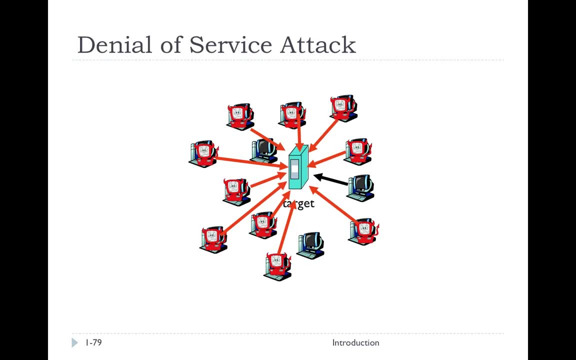 or bogus requests. That is, the attacker just trying to overwhelm you with these fake requests so you can't get any real work done. Uh, the idea is that we would select target, um, the bad guy would, um, possibly break into several other hosts. 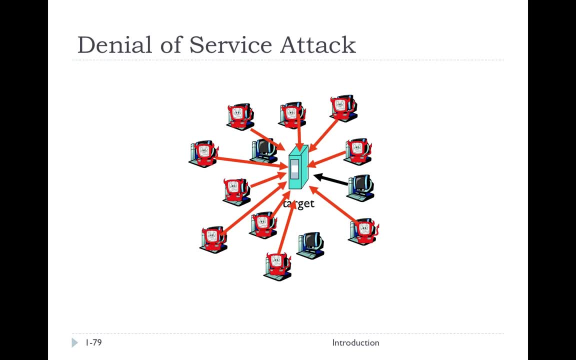 to have this big botnet and then have all of those hosts at the same time send packets requesting resources from um from this target server. So that's a denial of service attack and and perhaps even a distributed denial of service attack. 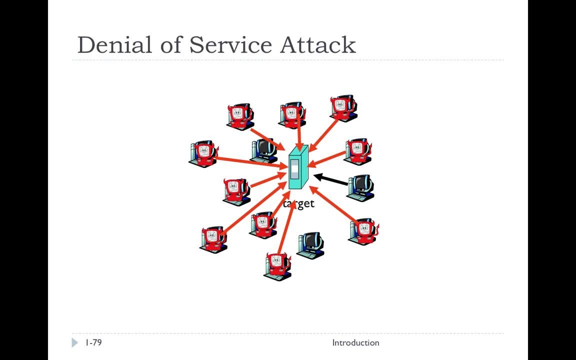 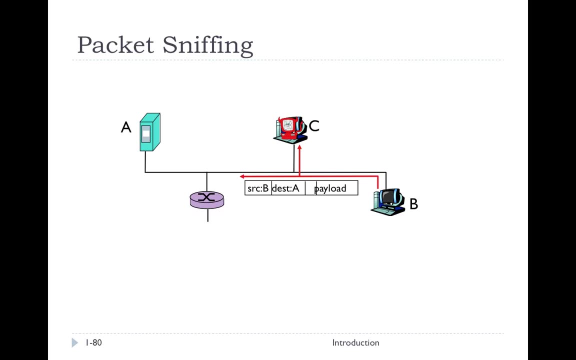 if lots of um distributed hosts are doing the attack. Another type of network attack is something called packet sniffing, something that we're gonna be uh using in our Wireshark Labs. The idea is many uh physical media are broadcast media. 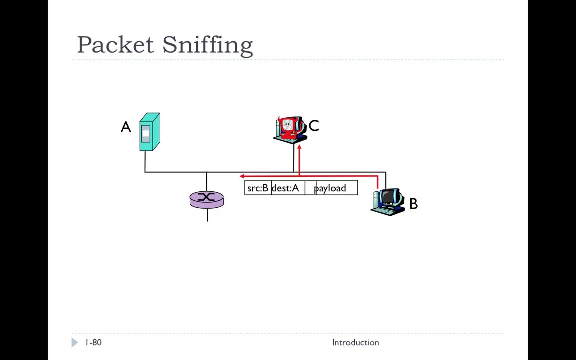 Things like ethernet and wireless uh come to mind. On a wireless network, everybody can hear what everybody else is saying inside um, that local area network. Usually you only listen to the packets that are addressed to you, but it's possible to um to get access to the packets. 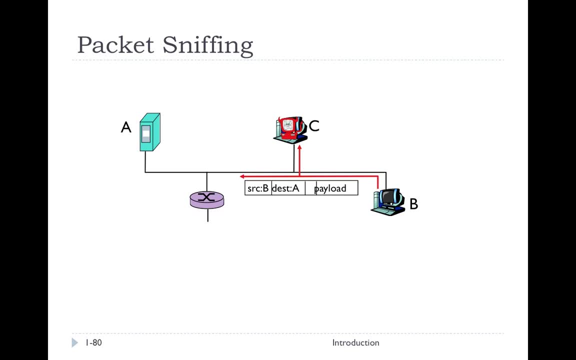 but it's possible to um to get access to the packets. change your configuration so that you listen to everything that's said, not just the stuff that's addressed to you. Malicious users then might listen for packets that are very interesting and record those things with passwords or other sensitive information. 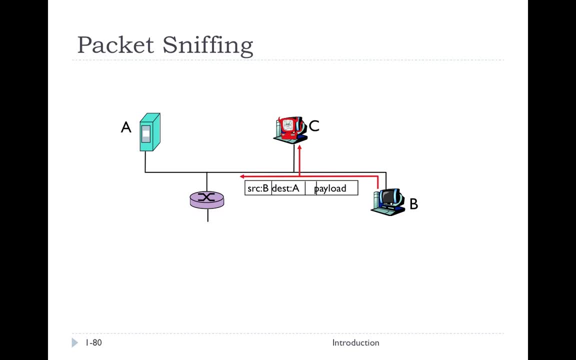 Wireshark is one free software, one free packet sniffing software that we'll use in our class to experiment and to learn about some protocols. Another type of attack is called IP spoofing. The idea here is that you can lie about your source address. 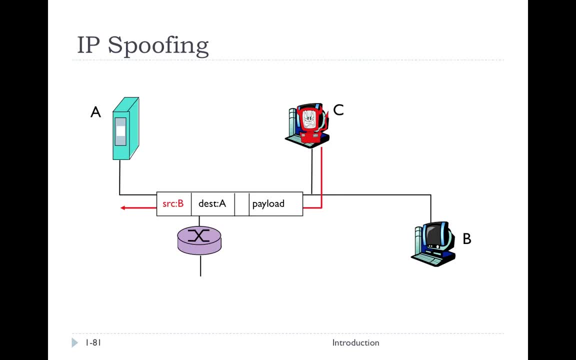 and pretend to be somebody else. You can spoof their address and even though you see C here, the bad guy, he's claiming that he is source B and sending a packet to destination A, but he's definitely not. So we need to have mechanisms in our protocols that would prevent this kind of spoofing. 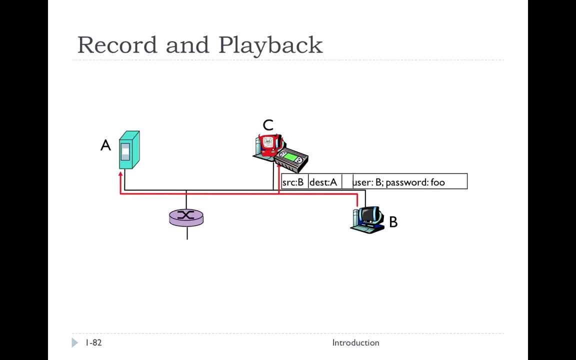 of your address and trying to impersonate somebody else Related to that, a record and playback attack. the idea is that you can sniff, that is, record, overheard sensitive information like passwords and such, and use them later by simply recording what you heard.